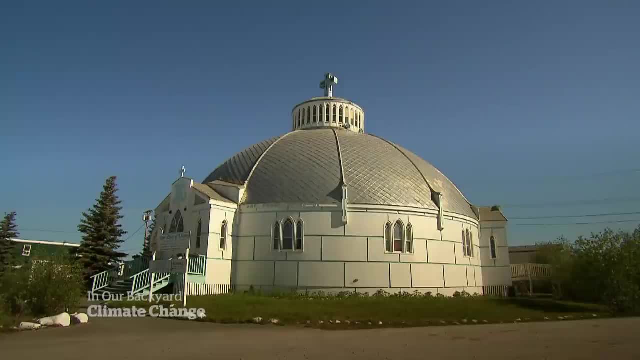 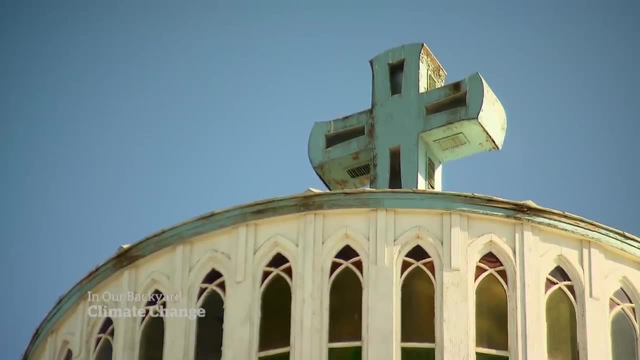 Holy cow Right. The Igloo Church, as it's called, was built on top of thick layers of earth and solid ice, But that concealed permafrost is now thawing, threatening the church's future. The Igloo Church's foundation. 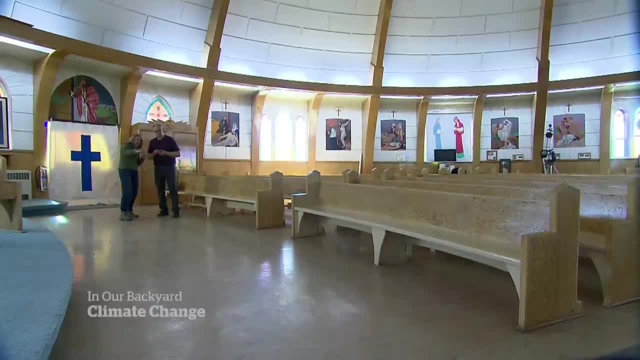 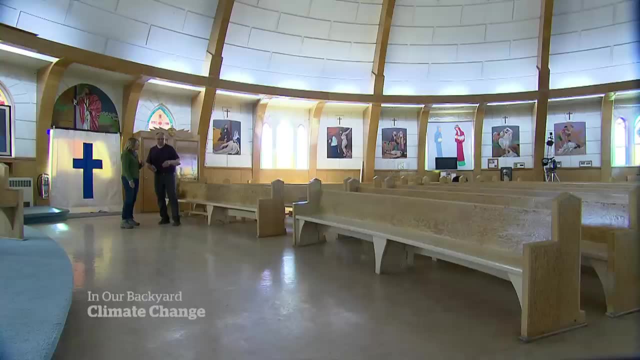 Joe standing here you can even see it's kind of sloping, Right? Yes, I'd say probably. it's down a downward slope of three to four inches minimum, maybe even more. Wow, Yeah, If I could roll a marble here. 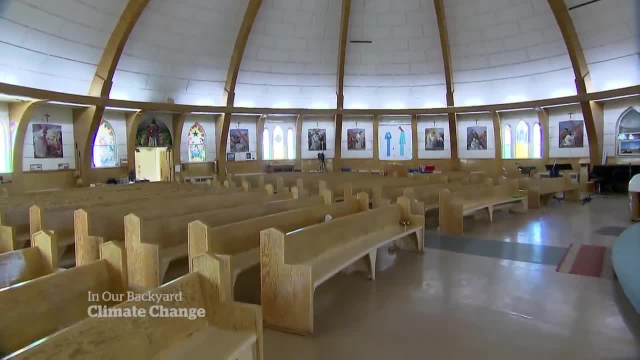 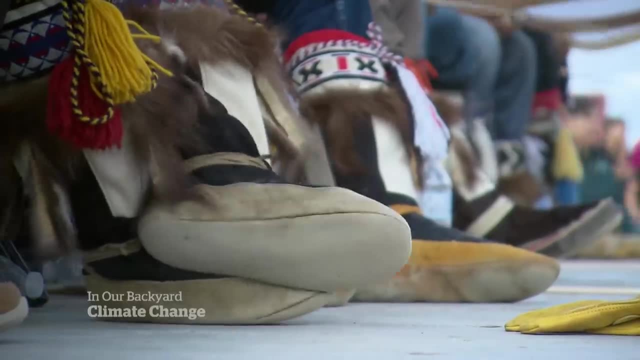 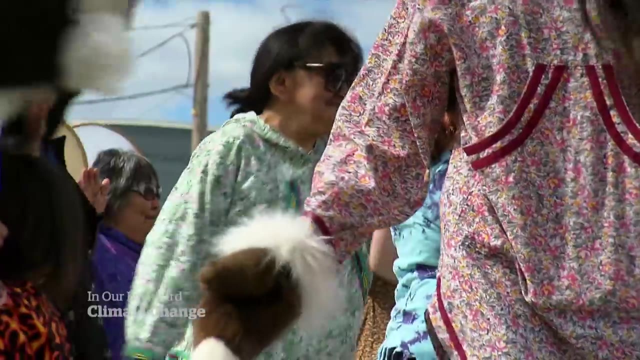 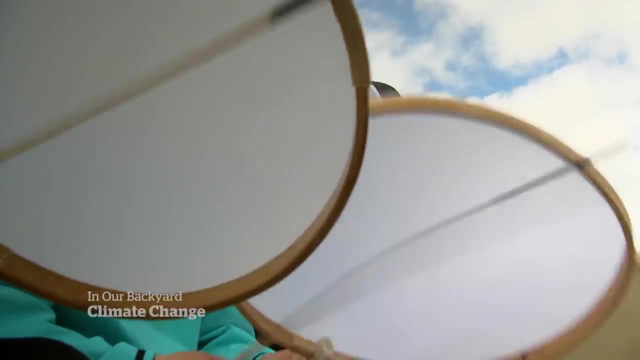 You sure don't want it to collapse? Absolutely not. Yeah for sure, that would be a real tragedy. The Inuvialuit have been living on ice for centuries, but the town Inuvik was only incorporated in 1961.. Tradition is baked into their culture, just like the certainty of 24-hour sunlight in summer and a dark, frozen landscape in winter. But ask anyone here: The Western Arctic is warming faster than anywhere else in Canada. Mean temperatures rise faster than anywhere else in Canada. Mean temperatures rise faster than anywhere else in Canada And rising a staggering 3.5 degrees over 50 years. 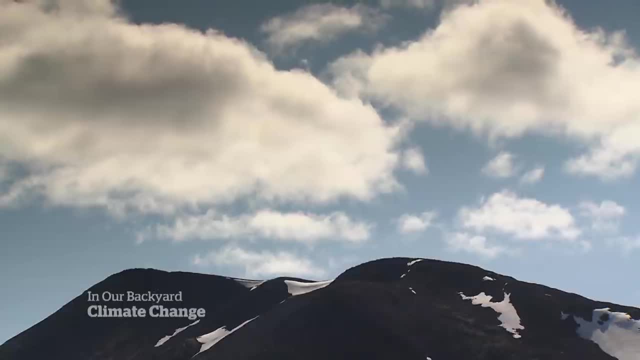 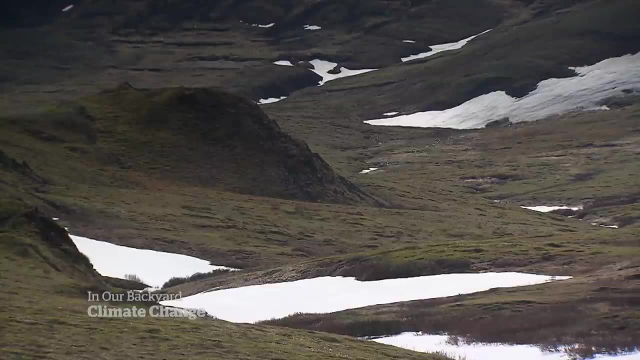 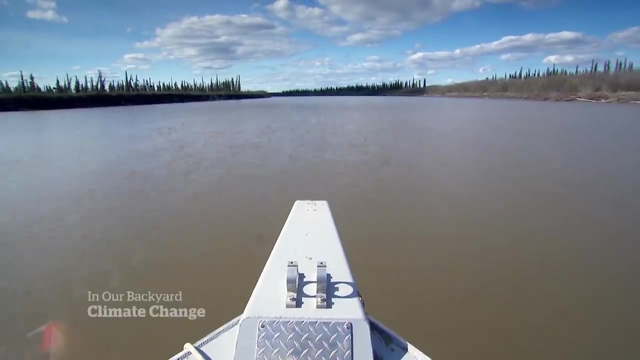 And rising a staggering 3.5 degrees over 50 years. Most of the Western Arctic is underpinned by icy permafrost And as it degrades, it's causing all kinds of challenges. A big river. The climate is not just warmer here, it's wetter. 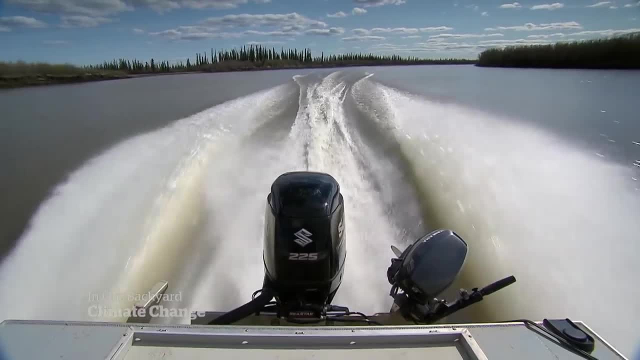 We're motoring up a branch of the Mackenzie River which in winter, is an ice highway. Chris Byrne has been coming up here for the winter. Chris Byrne has been coming up here for the winter. He's been here for 36 years. 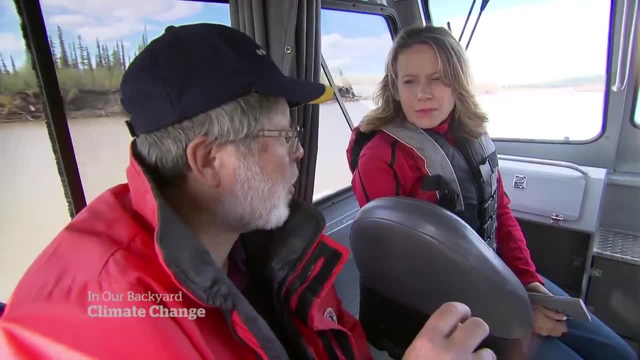 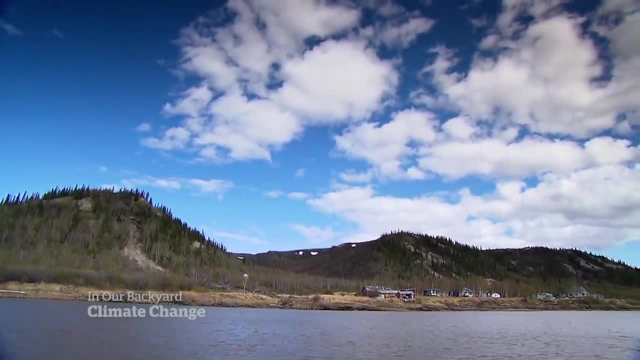 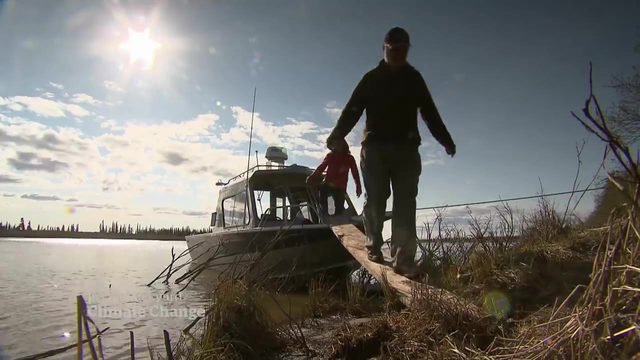 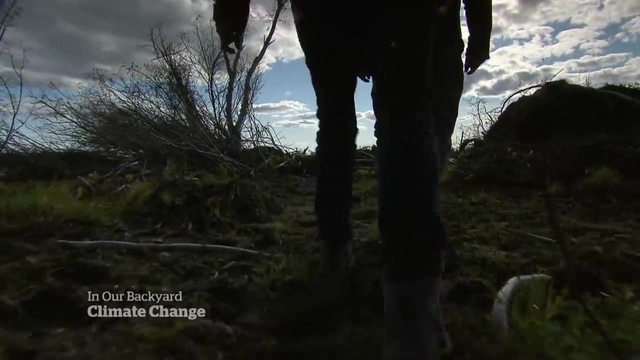 He's professor of geography at Carleton University and works with the Aurora Research Institute. Byrne wanted to show us the dramatic changes in the Caribou Hills at an old camp called Reindeer Station. First we have to navigate the landing. There's about 90 meters of permafrost below us here. 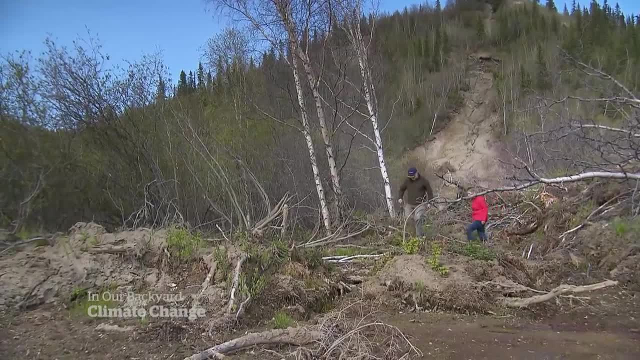 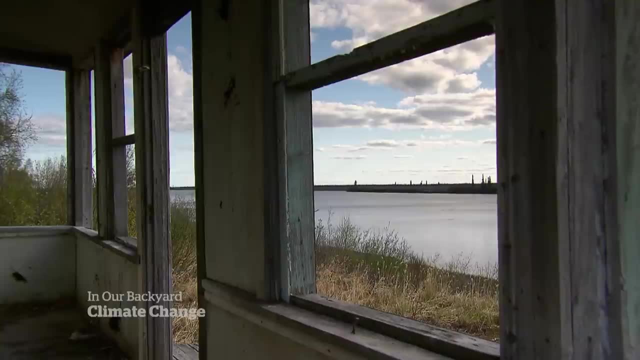 And some of that is thawing And the top of that is thawing. Years ago, this was a Hudson's Bay trading post, solidly built, like everything else, on buried ice, But that scar in the hill was recently carved by a landslide. 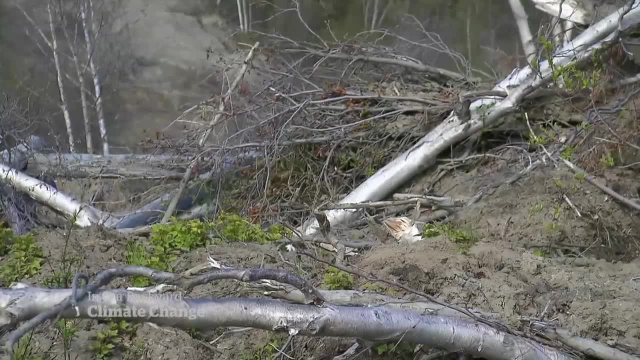 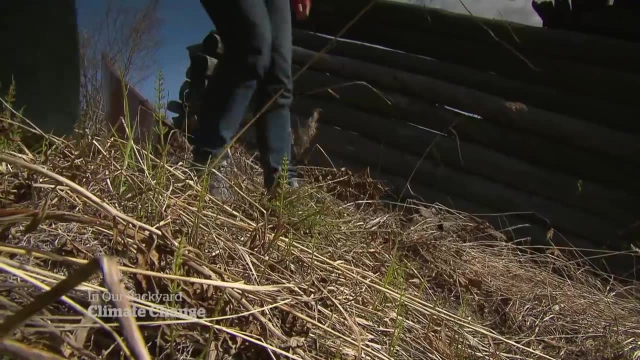 After heavy rain at the end of a summer, the warming earth simply gave way. This is basically where the landslide finished, And this wasn't the only one that night. No, no, no. There's 87 other landslides from that night in about 17 kilometers of hillside. 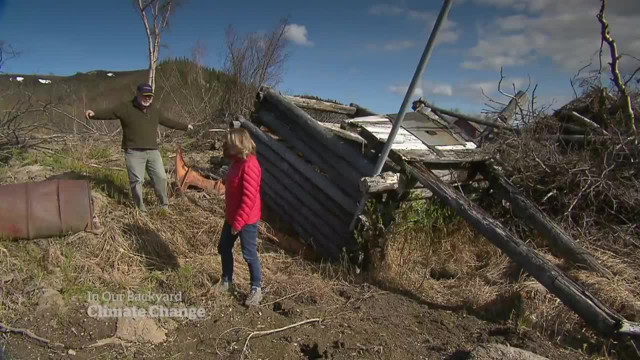 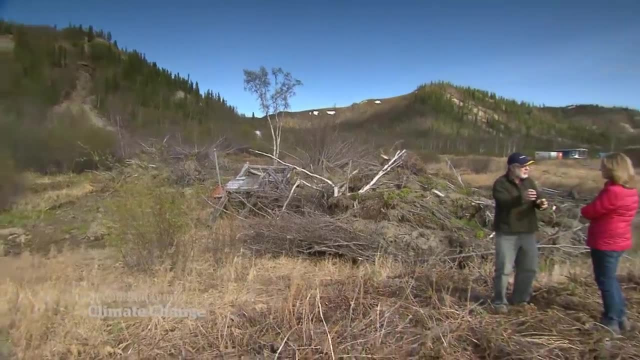 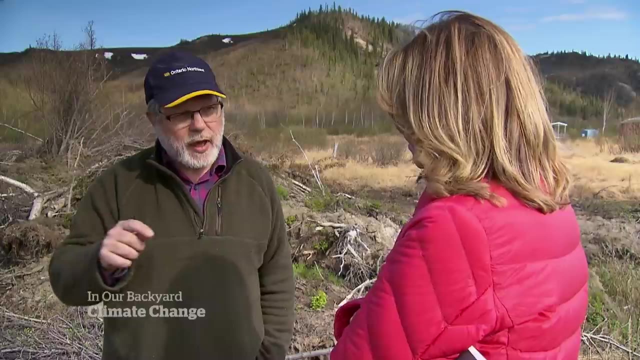 So it was a phenomenal event. This is a remote retreat now. No one lives here permanently, But the changing geography is the same in populated areas. We have to figure out what we're going to do in the future And we have no basis to believe that this will not continue. 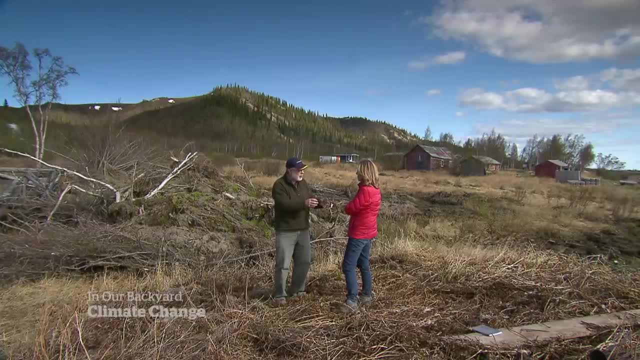 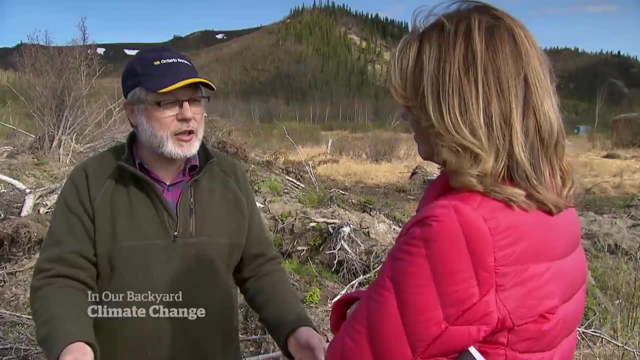 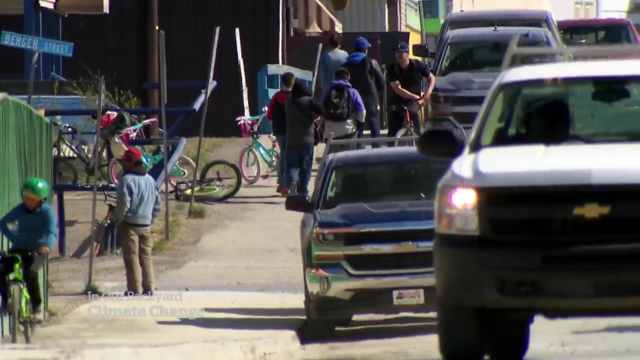 It won't stop now. So then, when we make an investment in a building which is meant to last 50 years, if in 15 years it's no good, we've wasted a huge amount of resources. Inuvik is adapting. 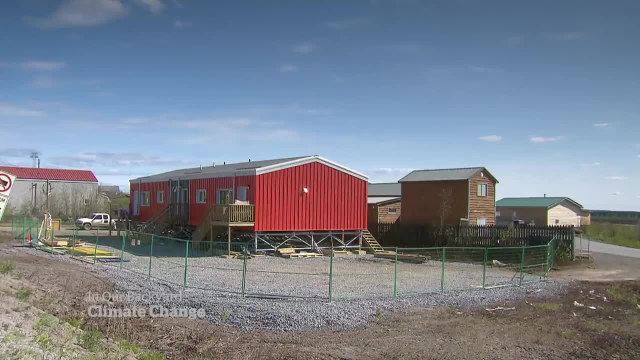 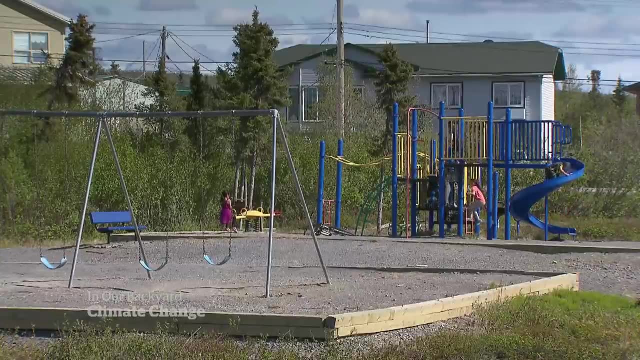 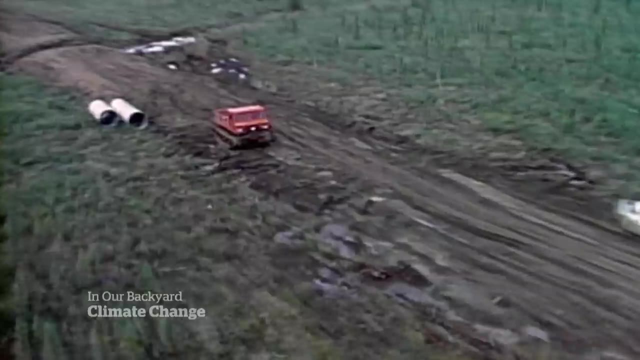 An above-ground sewer system is being retrofitted. Flexible space frames prop up some housing, But it is patchwork. Back in the 60s, when Inuvik was built, permafrost seemed a more reliable, solid core. We said we'd open roads into the north. 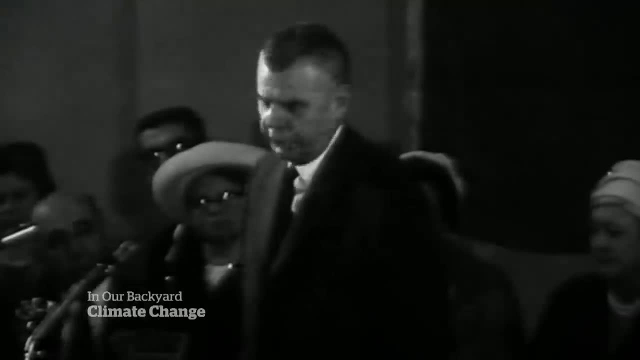 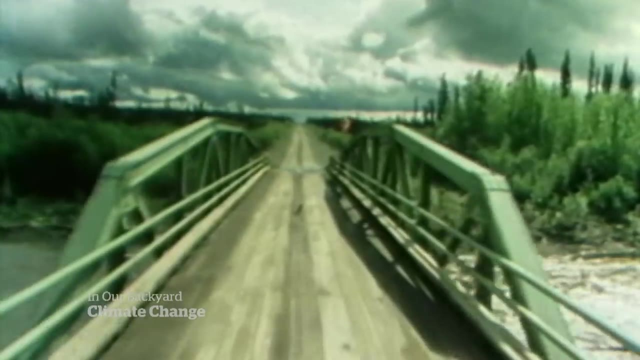 It was Prime Minister John Diefenbaker's dream: Resources should be made available to the people of Canada. A northern road linking southern Canada to the Arctic, A road to resources. The Dempster Highway finally opened in 1979.. A construction marvel. 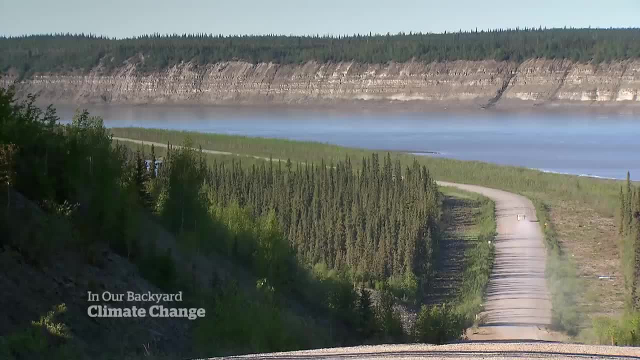 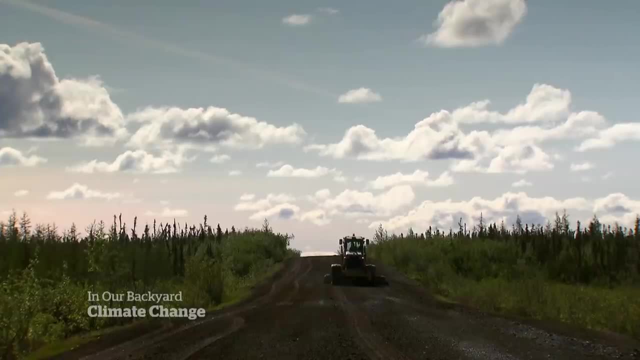 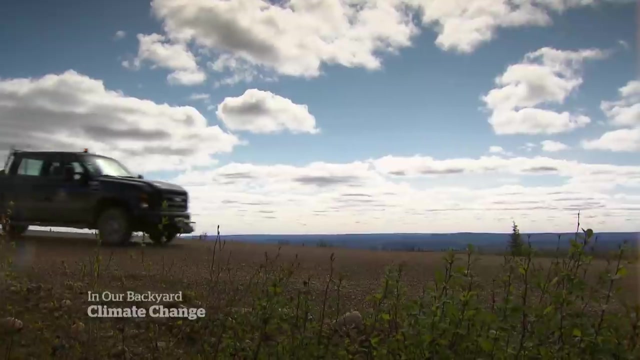 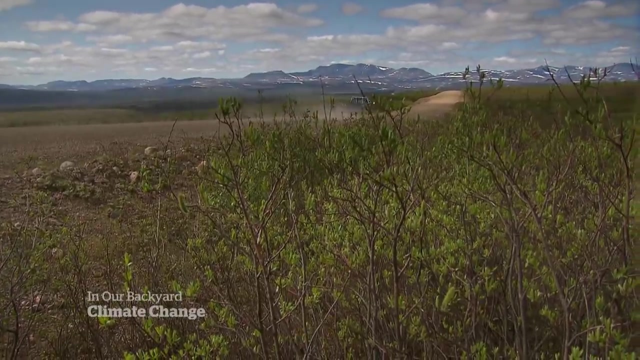 Over 700 kilometers of tundra Music, But every year it costs more to upgrade the highway. Climate change over the last 15 years has pushed up costs by the millions. It's kind of like the lifeblood of the Western Arctic. Steve Cookelle is with the Northwest Territories Geological Survey. 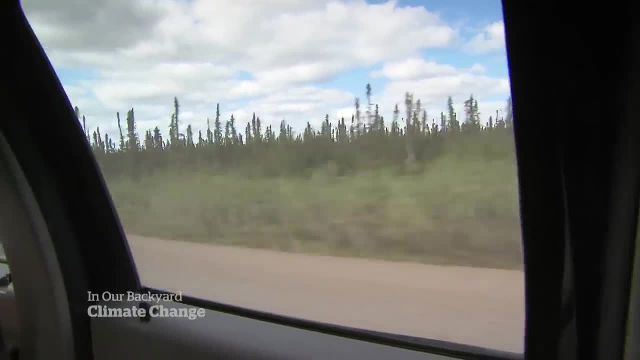 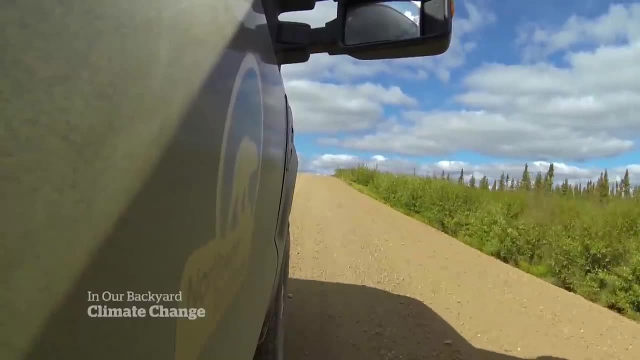 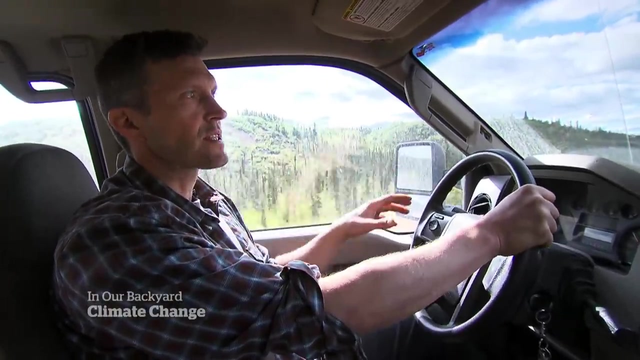 He's been up and down the Dempster for a decade. The Dempster Highway is built pretty much entirely over permafrost terrain, So the frozen ground beneath the road embankment provides a foundation for the embankment And the actual road itself has a frozen core. 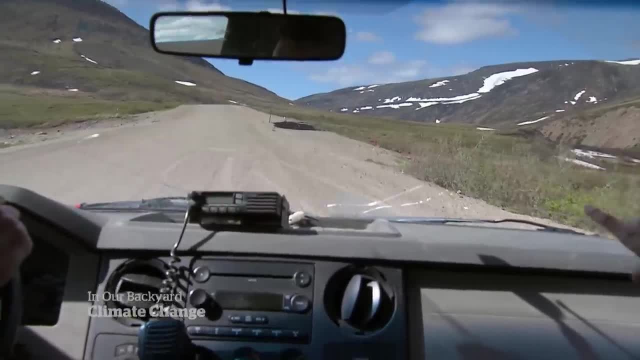 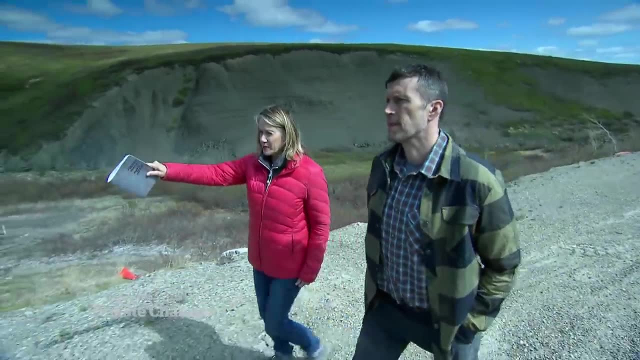 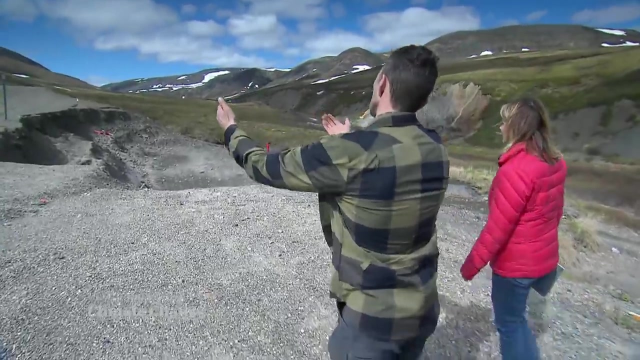 But this plateau is warmer and wetter now And the highway is showing fatigue So clearly, Steve, the Dempster is falling off here. There's a big hole in the side of the road. Yeah, this is a location. We have a slope where water is collecting along the side of the road. 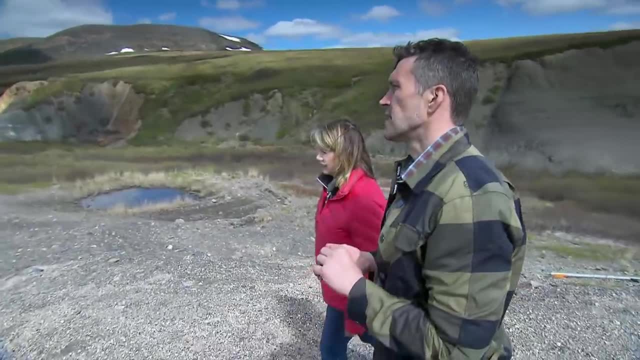 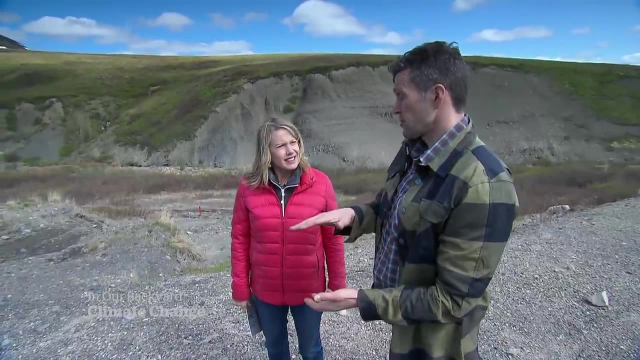 And the combination of warming climate, the impact of the road and the moisture is causing the underlying ice-rich permafrost to thaw. And as that ice-rich permafrost thaws, the ground consolidates or settles proportional to how much ice there is in the ground. 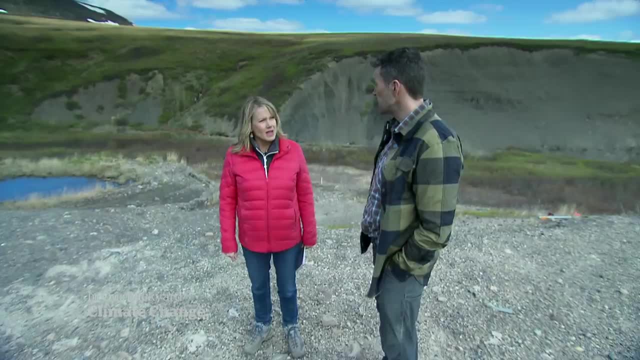 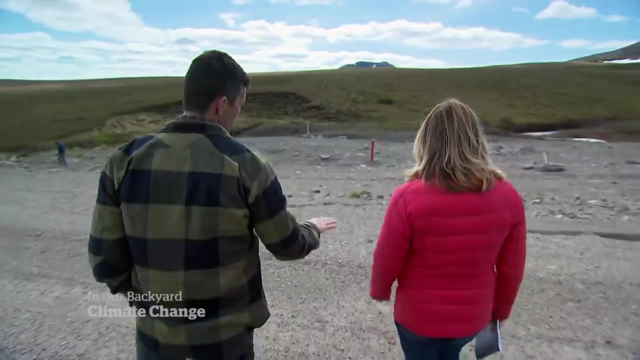 And this is one of the consequences of that. Now you told me that across here, this happened on the other side of the road first. Yes, Steve explains that load after load of gravel has been dumped into this subsidence just to keep the highway open. 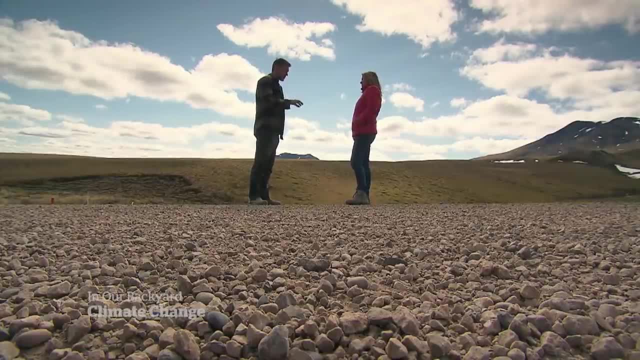 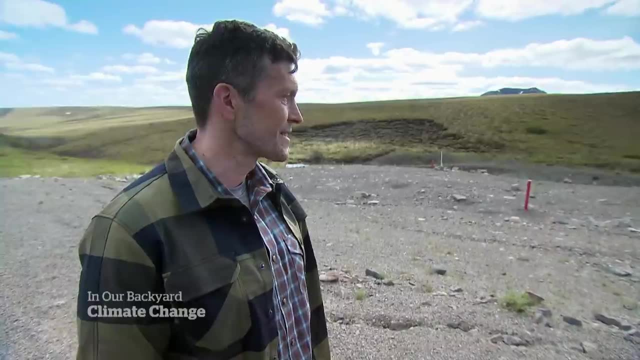 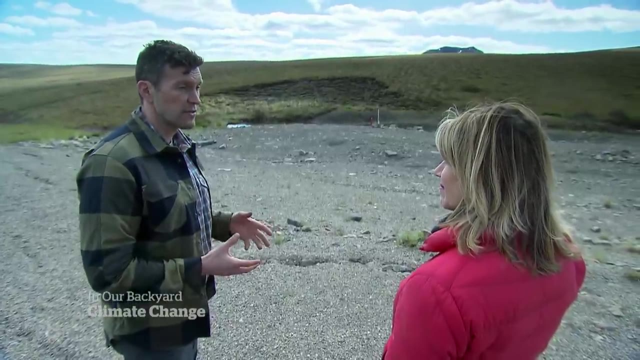 But it keeps sliding off, leading to a key question: Do we fix it or do we start to adapt differently? Yeah, I mean, I think that's a really interesting and important discussion. It really emphasizes or highlights the need to start to think innovatively about the solutions. 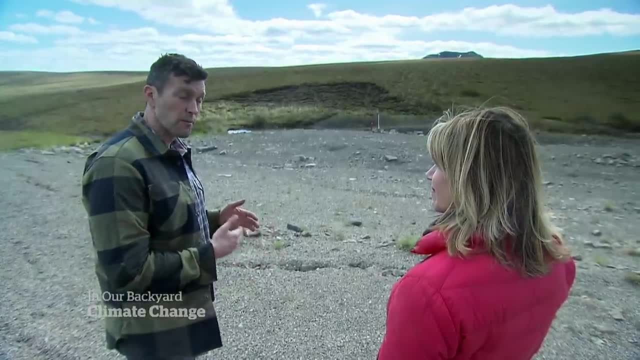 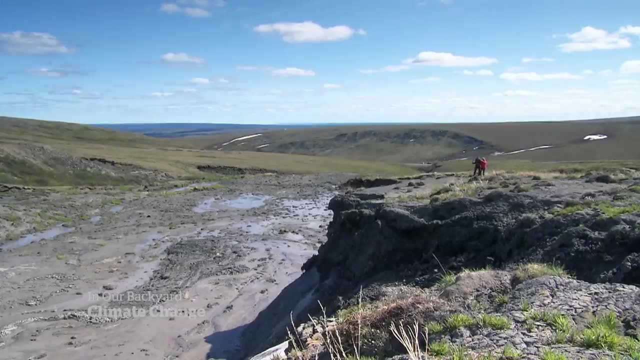 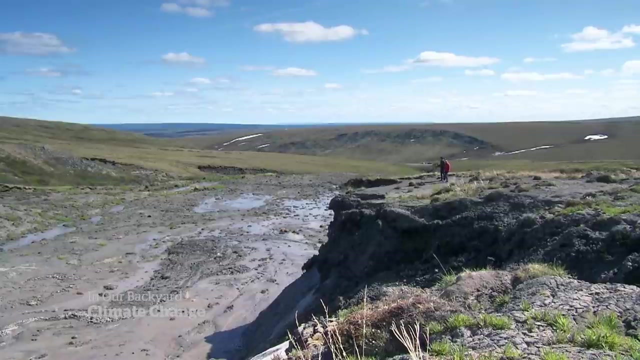 because these types of phenomena are going to become more and more commonplace. He's not finished our permafrost lesson. A few kilometers down the road, we clamber up to a high ridge. This whole area here has developed over the last couple of years, which is very, very rapid. 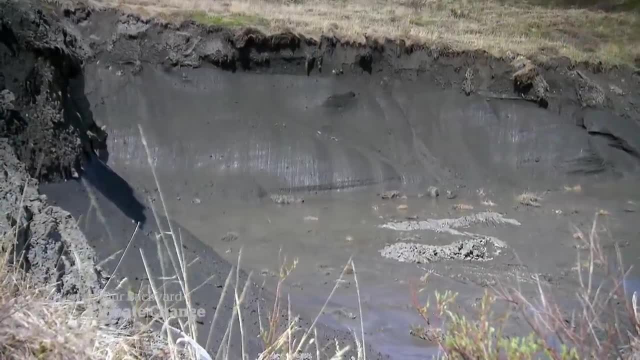 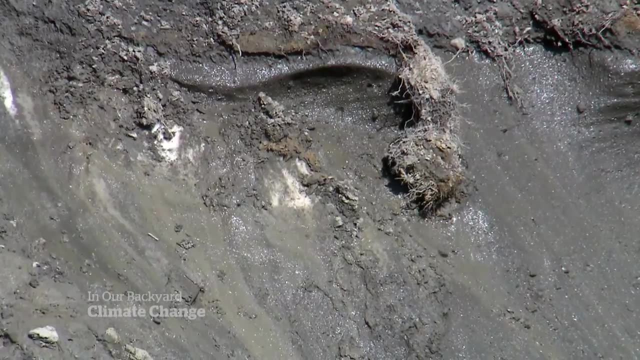 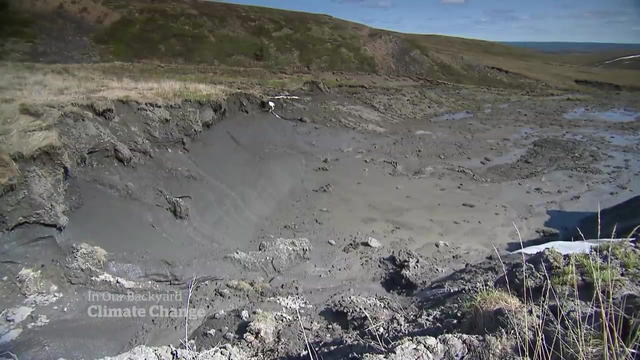 The headwall here has been carved out, exposing a wide band of ice. So the bottom five to eight meters is all ice. So that's what's thawing. That's exactly what's thawing. yeah, Constantly Recent thawing is creating a gully of mud pushing toward the Dempster Highway. 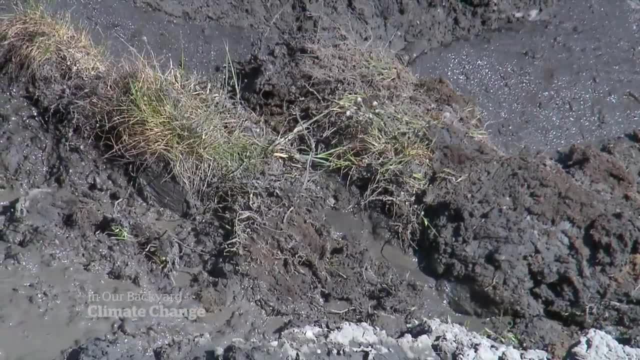 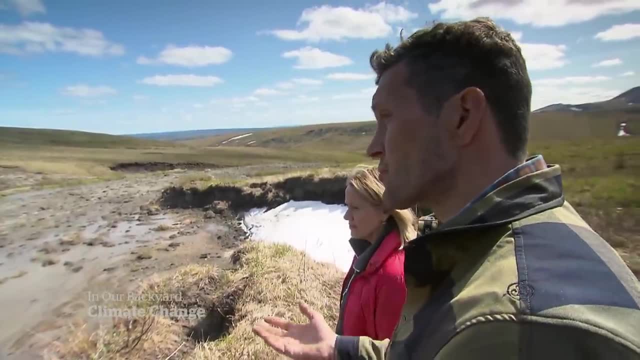 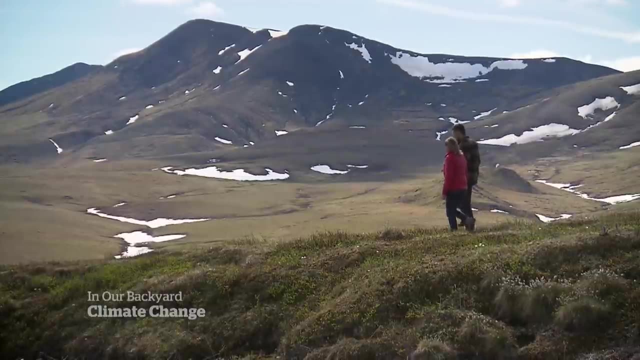 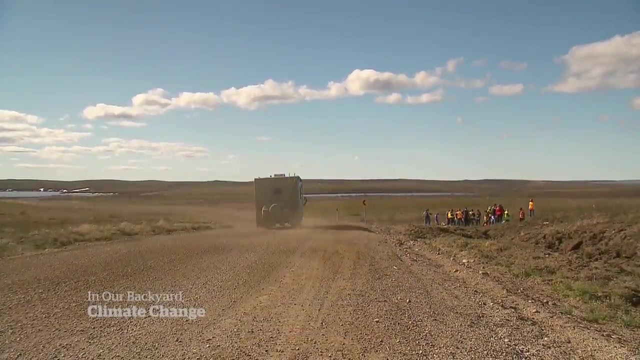 which in time could compromise the road. We've had this debris tongue that's grown about 150 meters towards the road That's developed in the last two years. Canada's permafrost problem has become a hot research environment. A recent Senate report identified northern infrastructure. 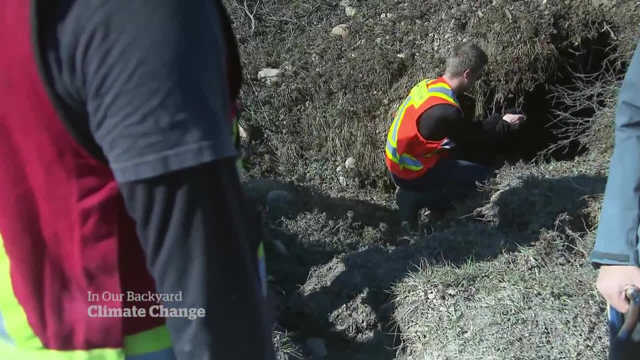 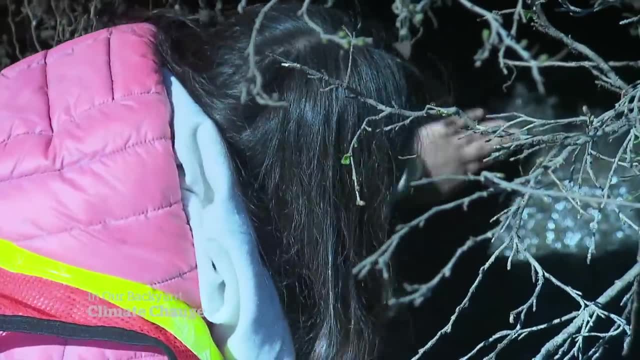 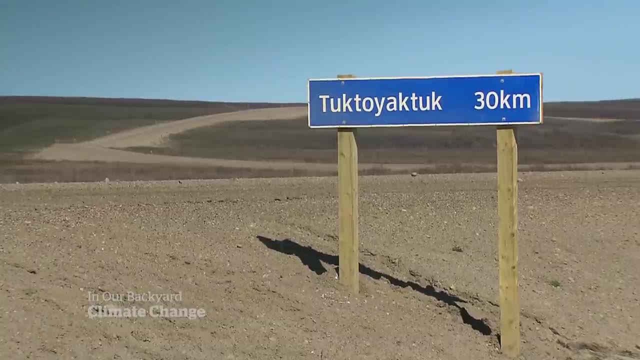 as an urgent priority. The challenge is luring international scientists and students like this university team on a field trip to study the ice under the tundra. Traveling further north on a new highway, we head towards Tuktayaktuk on the Beaufort Sea. 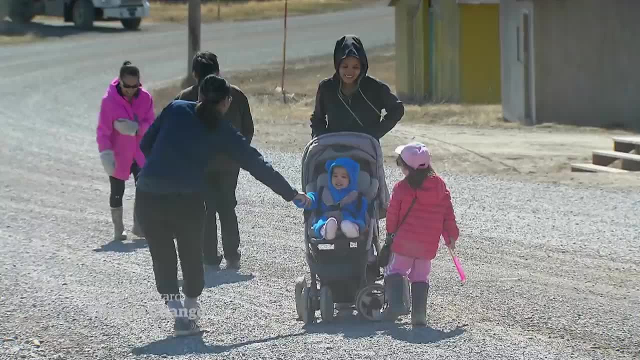 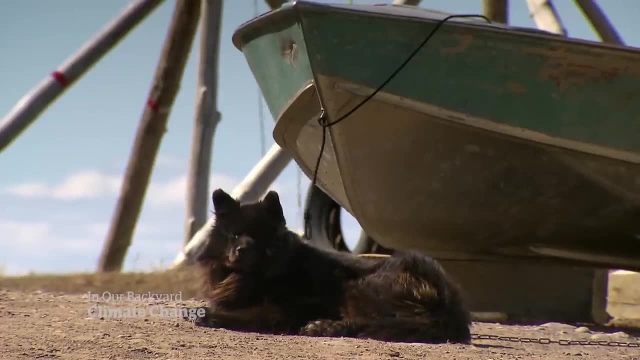 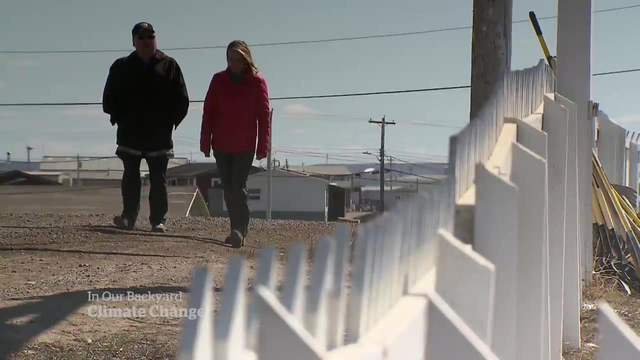 I made it to Tuk as a Traveler's Badge of Honour, but this hamlet has become a climate change crucible. Going forward, we're just not building anywhere near the coast anymore. We're slowly moving our infrastructure inland. Mervyn Grubin, the mayor of Tuk, grew up here. 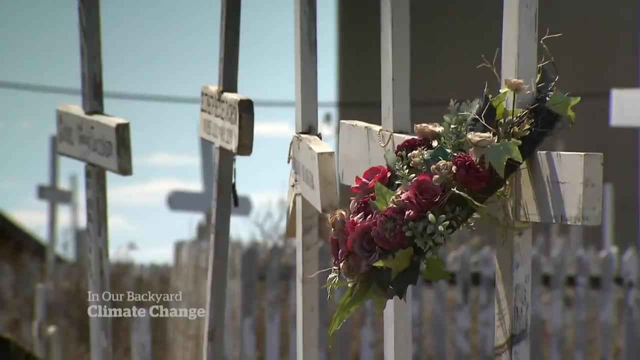 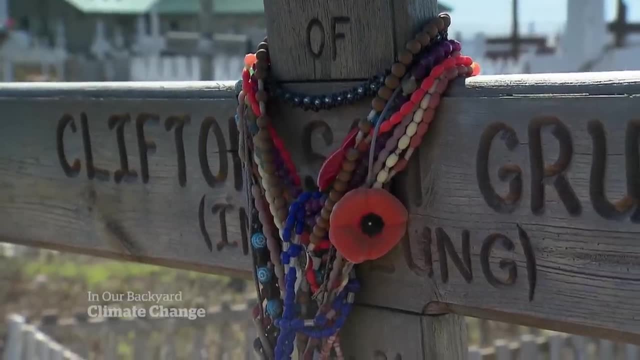 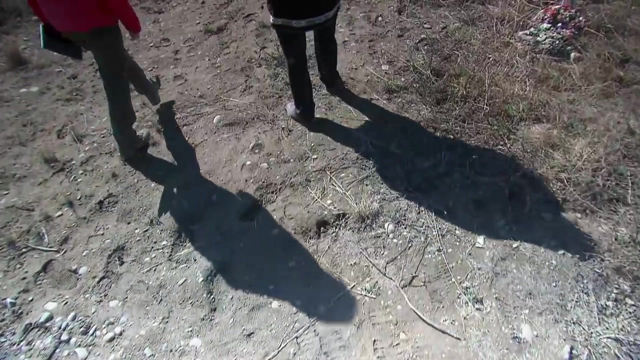 See all the ice. the land is melting Out on the point. Grubin's ancestors are buried now powerlessly close to the sea: My grandfather Edgar, My grandmother Mary. The cemetery's vulnerable: With more erosion it could fall into the ocean. 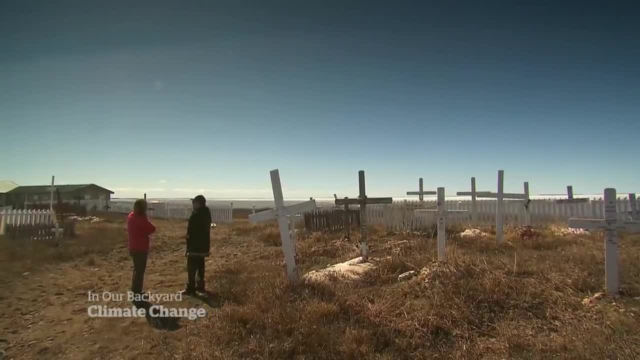 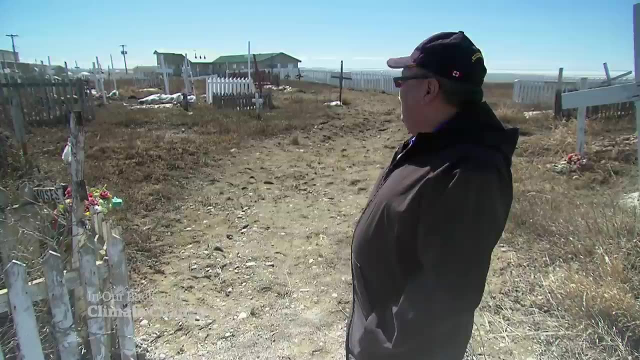 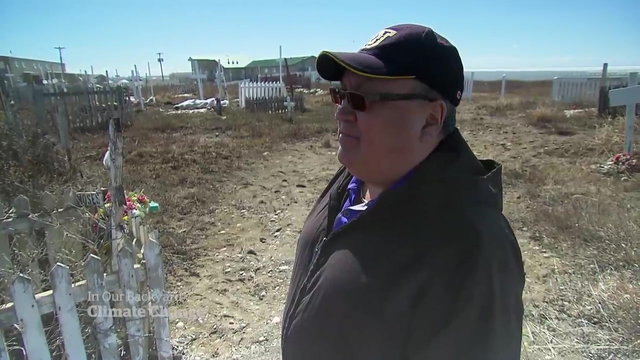 But moving graves is a last resort. I don't know, I don't know, Like the whole circumpolar north is sitting on permafrost. So what do you do? Oh, what do you do? You can't insulate the whole north. 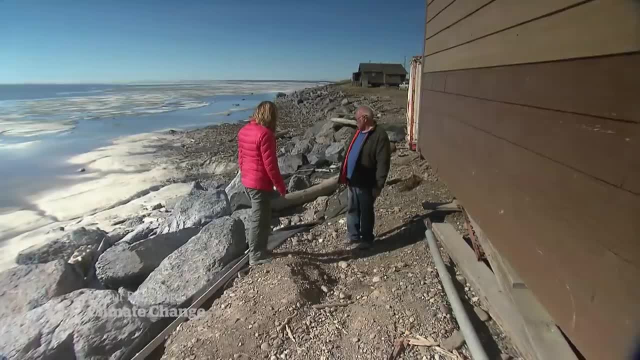 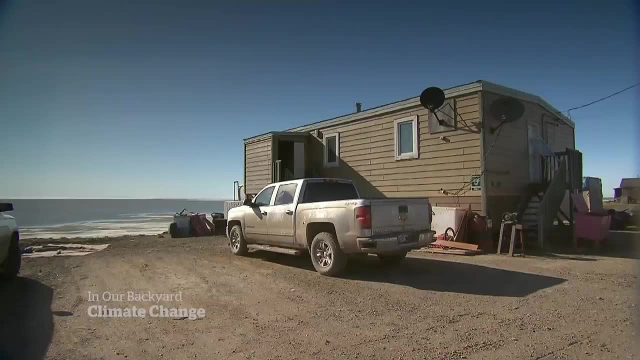 The dual threats of rising seas and thawing permafrost are undeniable. to Sandy Adam, a homeowner in Tuk, You could see the land eroding. His house is exposed right near the rocky edge. In 50 years he's watched that coast steadily erode. 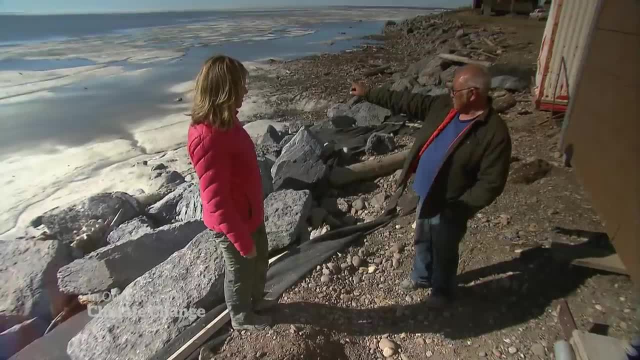 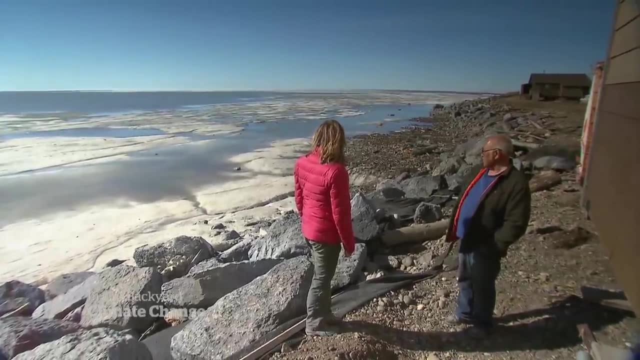 How far out did the shoreline go, Right to about the middle of the ocean, I mean where the open water is. That's how far the land used to be. Here it's really happening fast. We've got no time to waste. 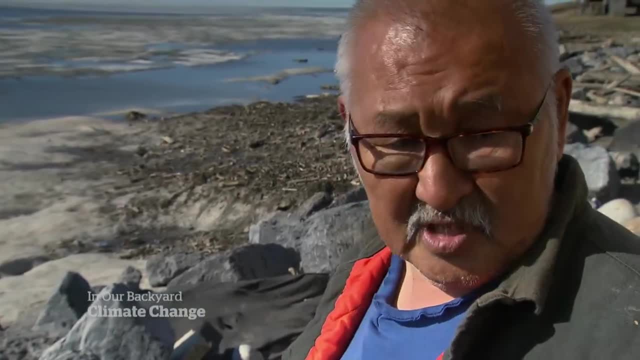 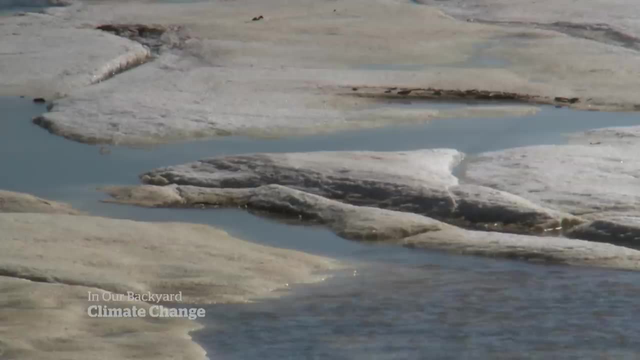 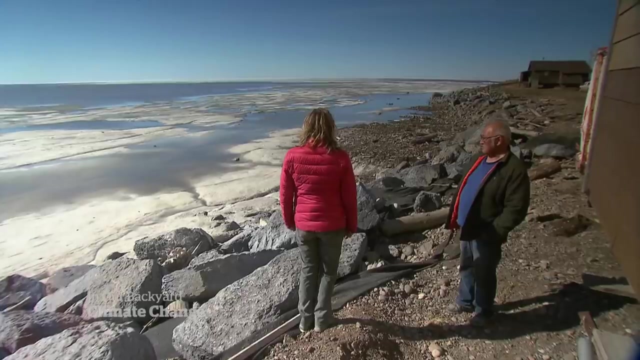 What do you fear? Well, I fear that my house can fall into the ocean. His house is on an emergency list to be moved inland. Five others already have. I guess they've got to move me. They've got to move me where I don't want to go but can't be helped.